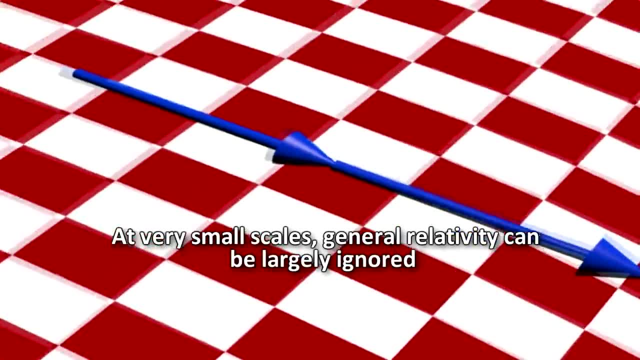 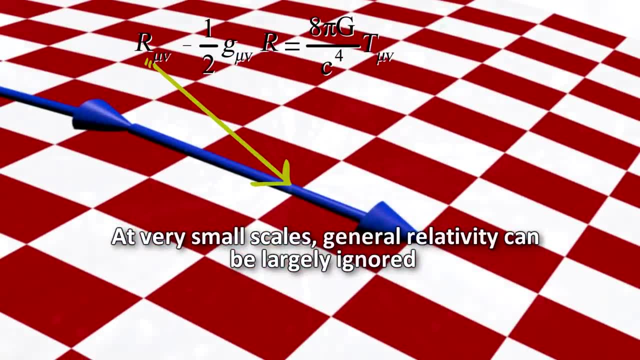 But this lack of success has not been a big issue for making predictions because at very small scales general relativity can be largely ignored because gravity has a negligible effect. 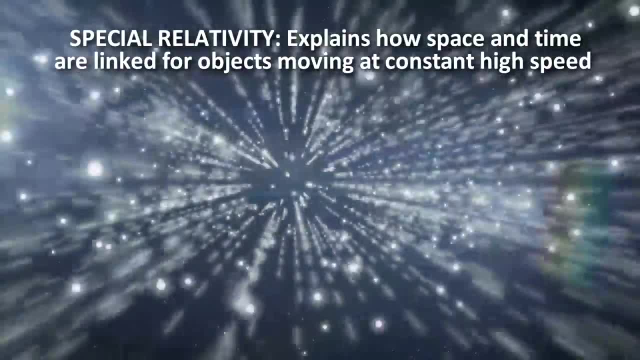 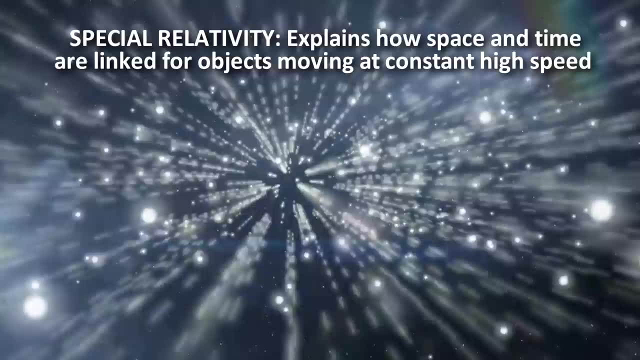 Things do move at very high speeds, and so to describe them at velocities near or at the speed of light, Einstein's prior theory, special relativity, has to apply. 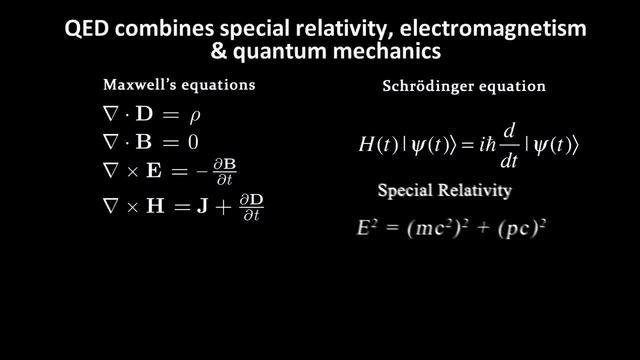 That integration of special relativity with quantum mechanics and electromagnetism is called quantum electrodynamics, or QED. 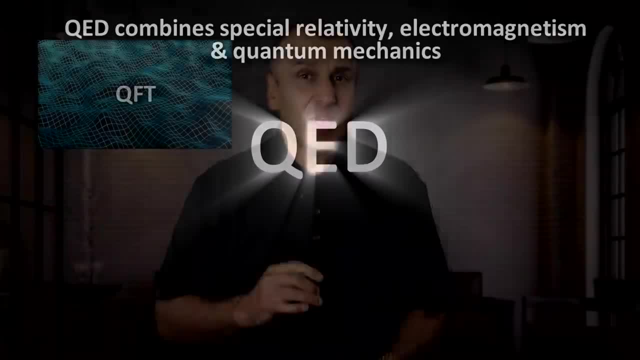 This is the most accurate theory man has ever come up with. Not only that, but it is also one of the most important concepts that led to the best description of the nature of the 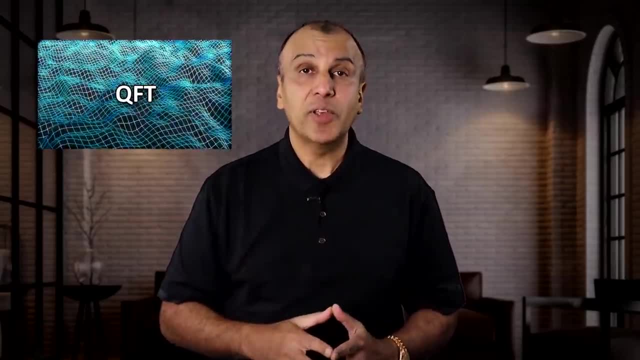 reality of the universe. And that is quantum field theory. 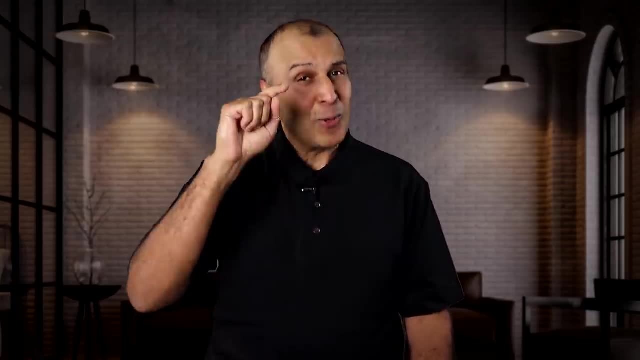 What is QED and how does it work? That's coming up right now. 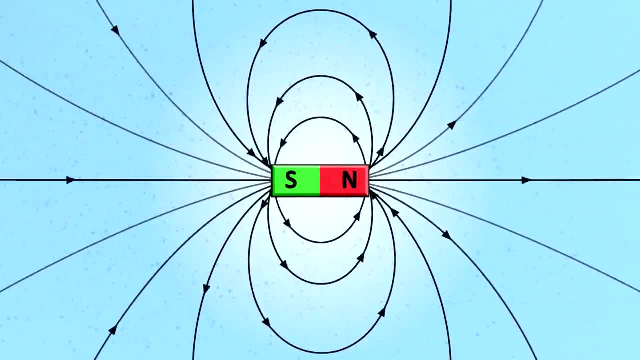 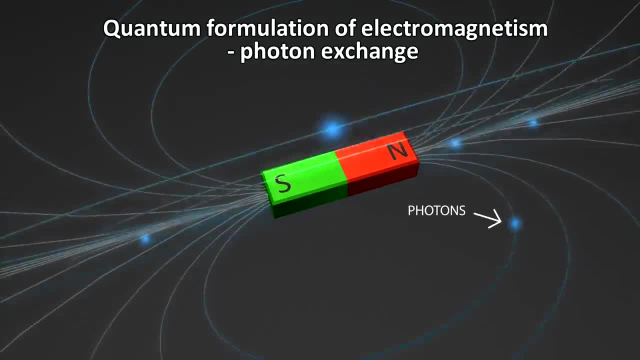 What QED does is replace the classical theory of electromagnetism, which involves continuous electromagnetic fields and puts them in terms of discrete quantities, a quantum formulation. 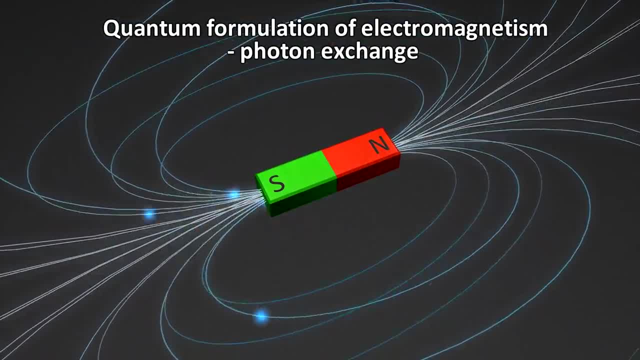 The idea is that small things such as electrons and other subatomic particles can go very fast. And when they do, special relativity has to apply. 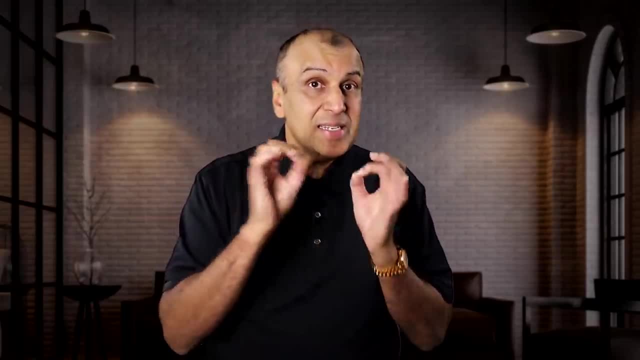 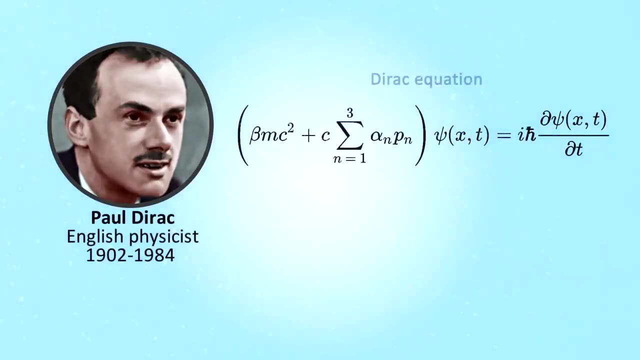 Many scientists over the decades helped develop the theory of QED, but in 1928 the first big step towards this unification was taken by British physicist Paul Dirac, when he published 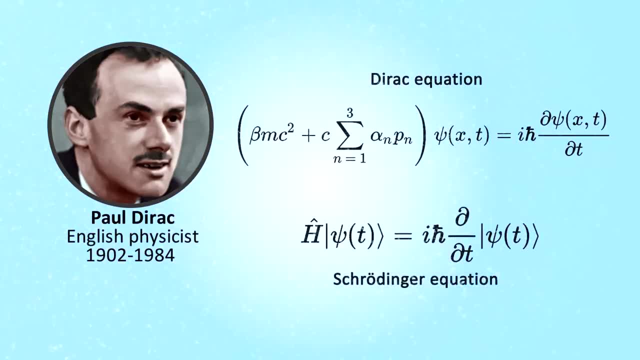 the Dirac equation, which blended quantum mechanics and special relativity. 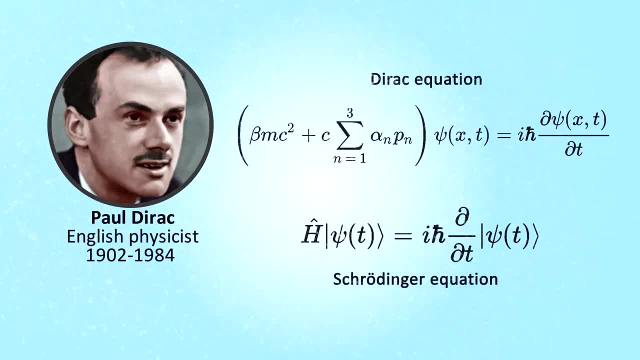 Notice how similar this equation is to the Schrodinger equation. Psi, which is the wave function, is present in both equations and indicates that this is a quantum equation. 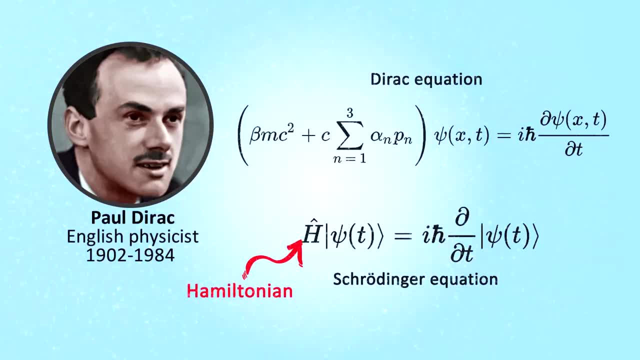 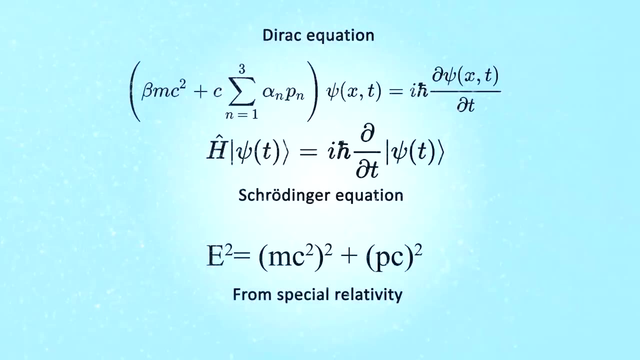 Dirac made a Hamiltonian, which is the sum of all the energy in terms of spacetime. And this signifies how special relativity is integrated into the equation. Notice the terms mc squared and p, the momentum on the left side. This comes from special relativity. It represents energy. This equation says that the rate of change of the wave function with respect to space and time, or rather spacetime, depends on the energy of the fermion. It's like the Schrodinger equation, except that it evolves in spacetime. 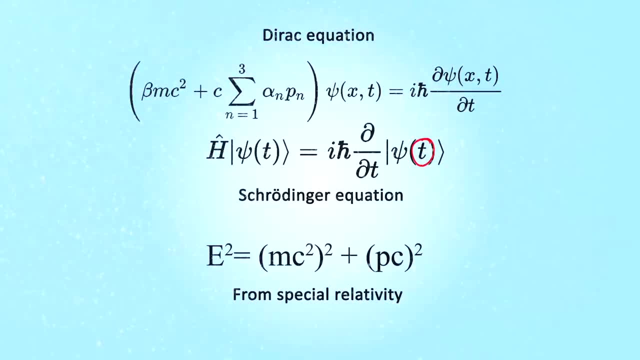 The Schrodinger equation treats time and space as independent coordinates, but Dirac integrates spacetime into the equation as shown by the terms x and t, as the coordinates of the wave function. 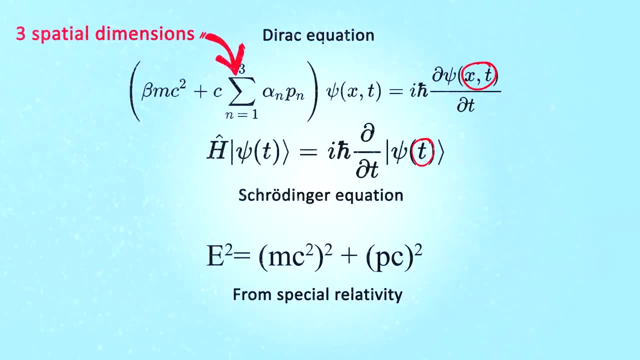 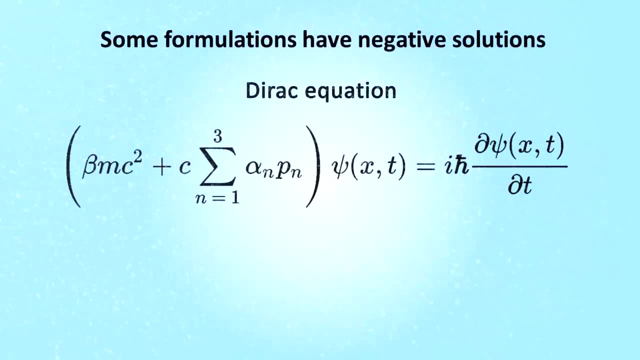 x represents the three spatial dimensions and t of course is time. One of the remarkable things about this equation is that there are some formulations that result in negative solutions. Negative solutions are not uncommon. You can simply use a number of ahh and then you have an infinite number of ahh processes. 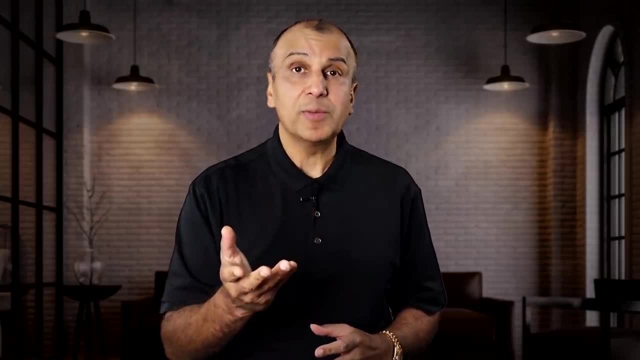 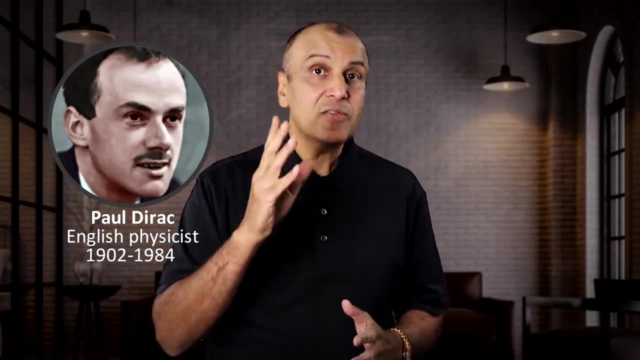 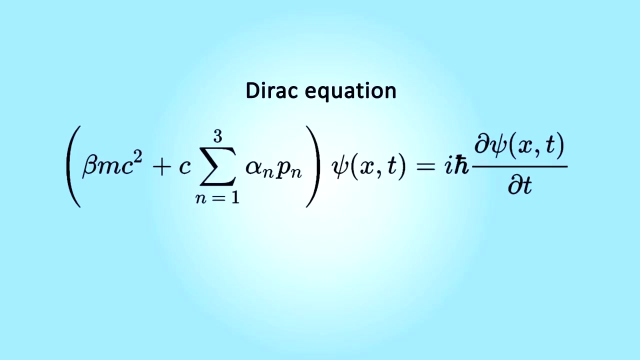 conviction. He believed his equation was so accurate that negative solutions had to be considered as a reflection of reality. His equation was predicting antimatter. No one had ever thought of that before. Dirac took the bold position of insisting that antimatter had to exist based simply on the math of his equation, with no experimental data. Notice the negative and 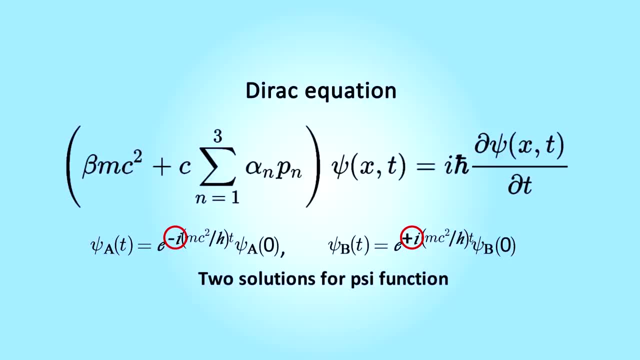 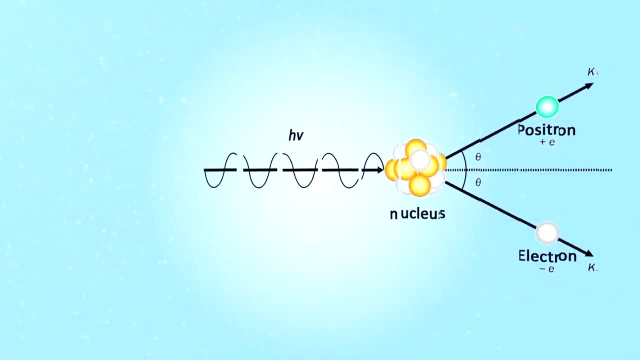 positive exponent solution of the function psi. That's where the idea of antimatter and matter comes from. Sure enough, four years after Dirac published his equation in 1932, the positron, which is the antimatter equivalent of the electron, was indeed discovered by American physicist 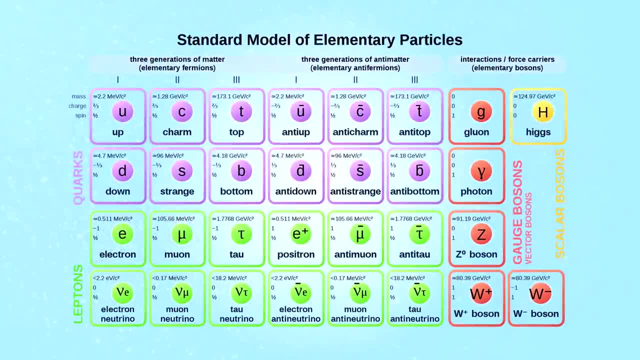 Carl Anderson. Today, we know that not only the electron, but all elementary particles have an antimatter equivalent. 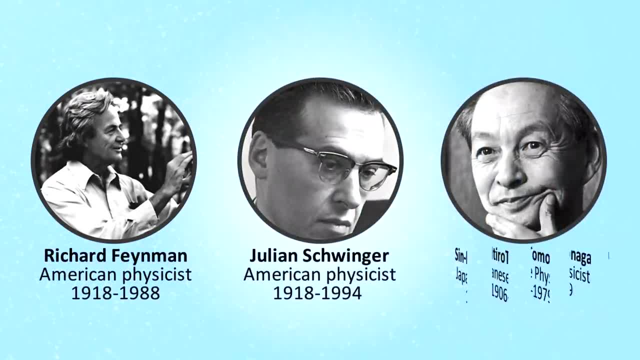 Later in the 20th century, three scientists began formulating a quantum theory of electromagnetism based on Dirac's equation, and formulated the central concepts of QED. These scientists were Richard Feynman, Julian Schringer, and Sinitero Tomonaga. They were awarded the 1965 Nobel Prize 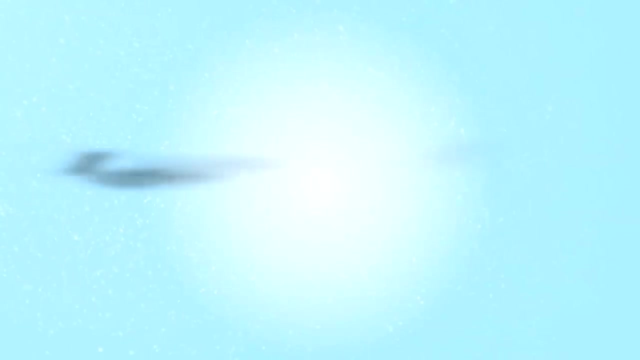 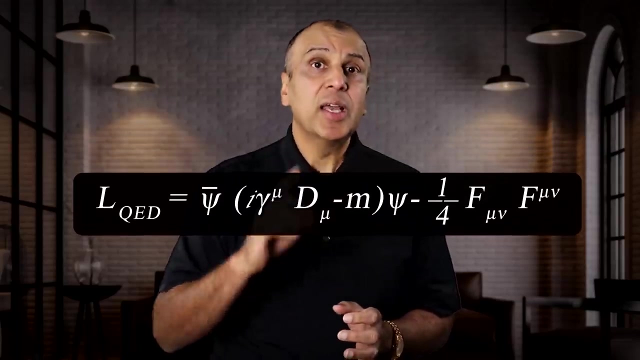 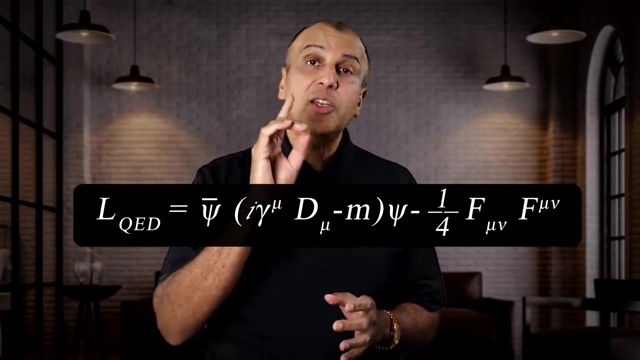 in Physics for their efforts. The result was the following. Here's what they came up with. This represents the Lagrangian, or the main equation for QED. Lagrangian contains all the elements of the equation. It contains all the energy terms of the theory. In other words, it contains all information relevant for the theory. And from this Lagrangian, you can obtain the behavior of the electromagnetic forces. Now, don't let this formulation intimidate you. I will explain intuitively what it means. 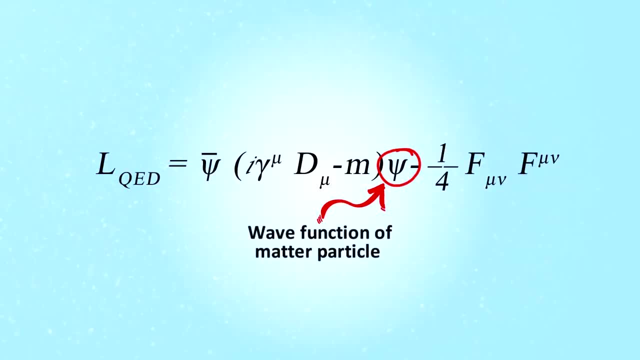 First, we can identify psi, that represents the wave function of the spin one-half field, 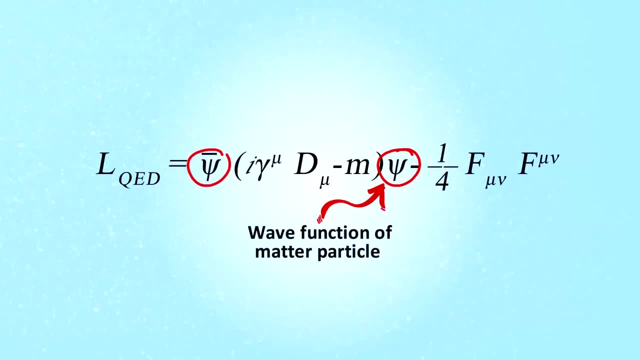 like the electron or positron field. Psi is the particle, and psi-bar is the antiparticle. The Lagrangian describes all the energies of the system. 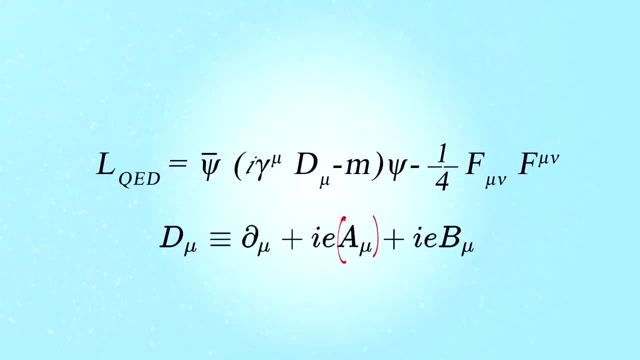 The fermion field, represented by psi and psi-bar, is coupled to the photon field, which is contained in the A sub mu, which is part of D sub mu. I gamma mu D sub mu contains information about how fermions, like electrons, interact with 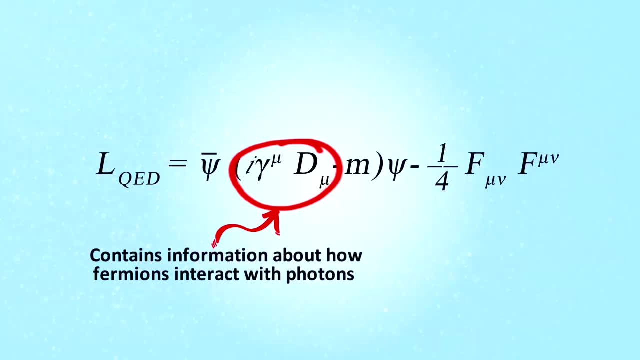 photons. In other words, how they interact with the electromagnetic field. And this is important for deriving the Feynman rules, which we're going to get to in just a second. 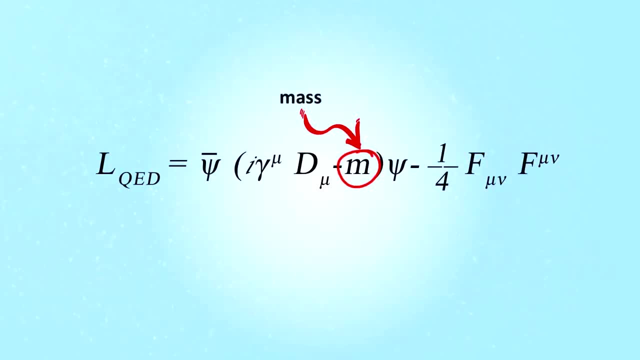 The m is the mass of the particle, like it could be the electron mass. The last term contains the electromagnetic field tensor, which contains the photon field and the relevant information about the electromagnetic field. This term basically contains Maxwell's equations. 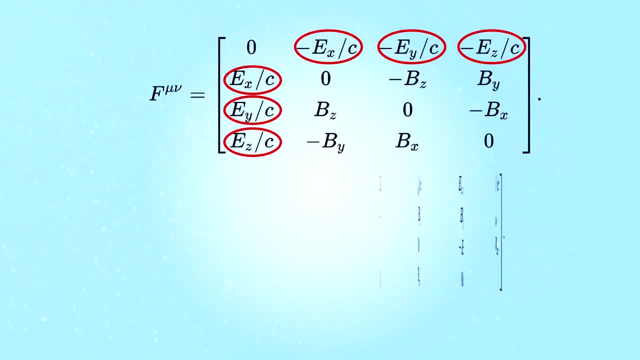 The difference between F sub mu nu and F superscript mu nu is a flipping of the electric field in opposite directions. 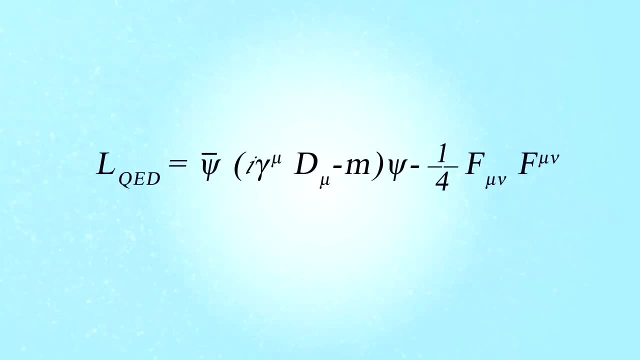 The formulation here gives us all the expected properties of the electromagnetic forces in the system. 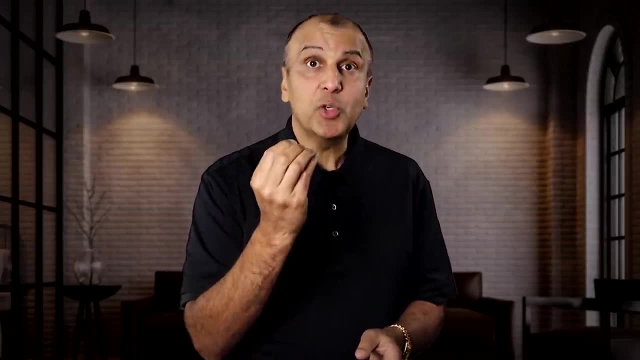 So now that you've seen the math, let's show what happens more intuitively. 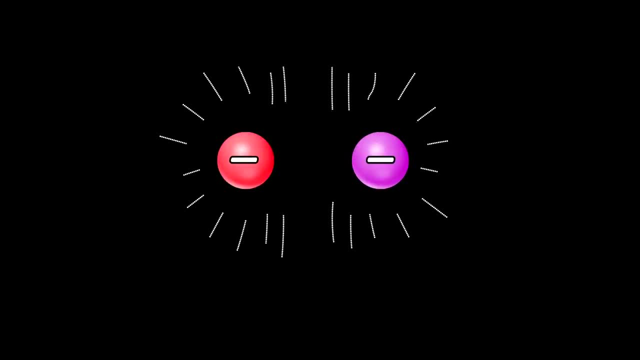 In the 19th century, it was thought that two electrons near each other would simply repel each other without ever touching, similar to the way the two like poles of a magnet repel each other without ever touching. 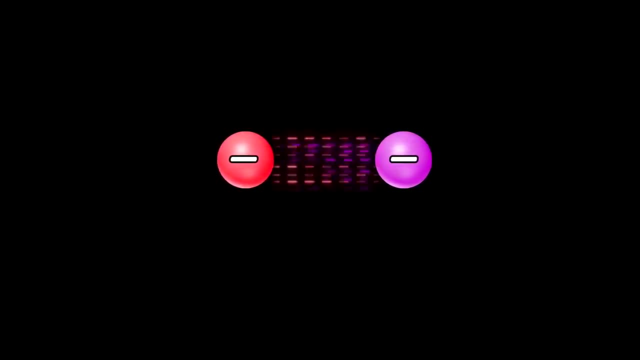 Paul Dirac and others showed that what is really happening is that there is no continuous field, but rather the forces are mediated by the exchange of discrete photons. They are emitting and absorbing photons, which results in attraction and repulsion. 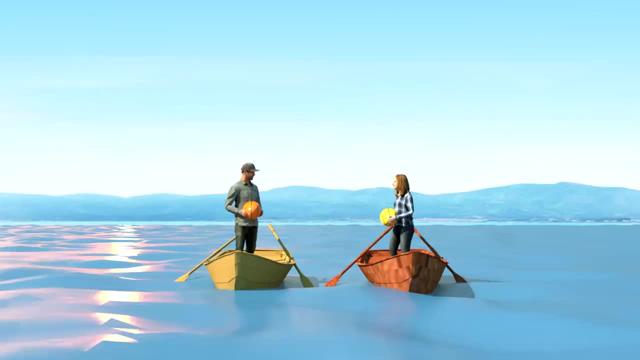 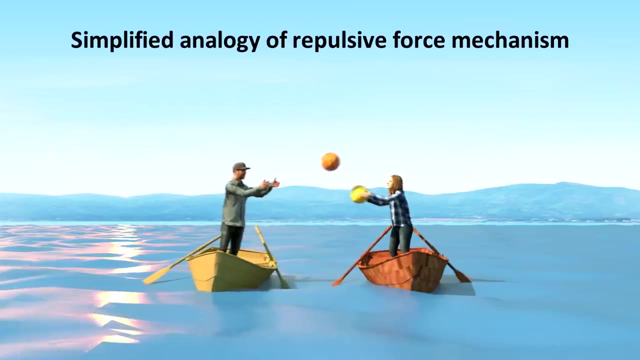 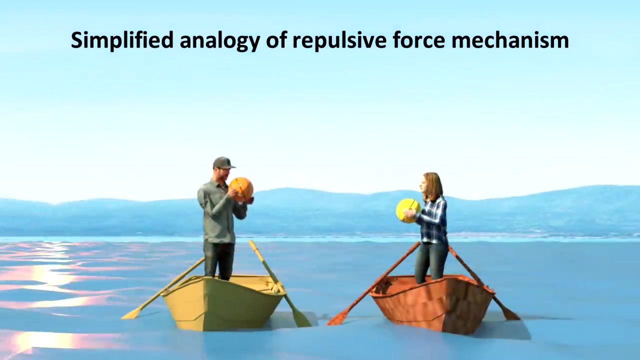 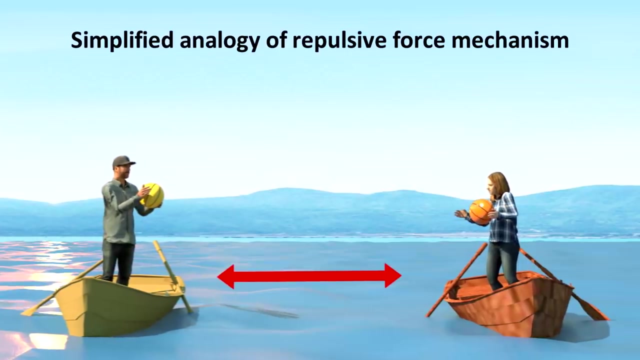 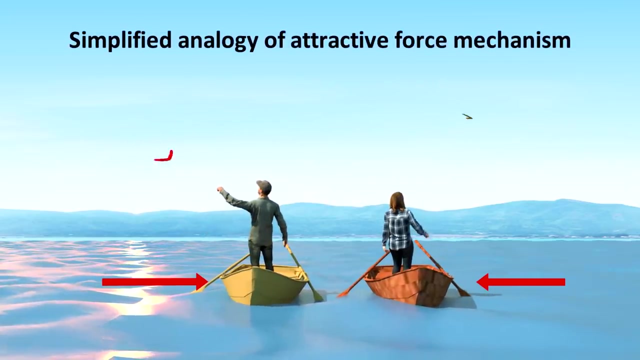 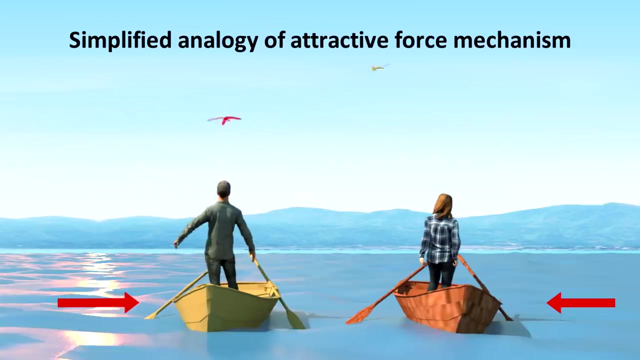 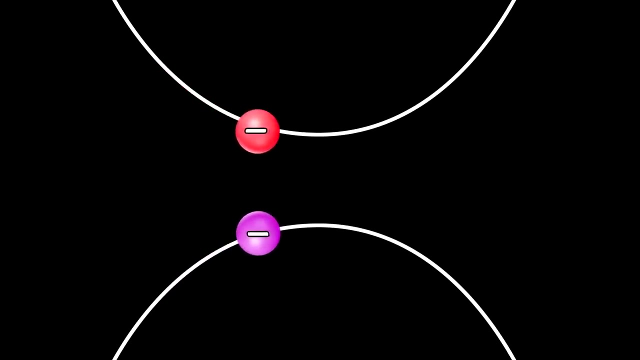 Here's a simplified analogy that I've used before. Think of two people on a boat throwing basketballs at each other. The basketballs are analogous to virtual photon exchange. The exchange of momentum of the basketballs results in the two boats moving further apart. This is analogous to how an exchange of virtual photons can confer momentum that makes two like charges move apart. Similarly, the exchange of negative momentum can occur analogous to two people throwing boomerangs away from each other. This is analogous to the mechanism of negative momentum exchange through virtual photons between two dissimilar charges. With this picture in mind, let's imagine two charged particles that travel near each other toward a colliding path. When they get close, they will repel each other and take a path that looks something like this. 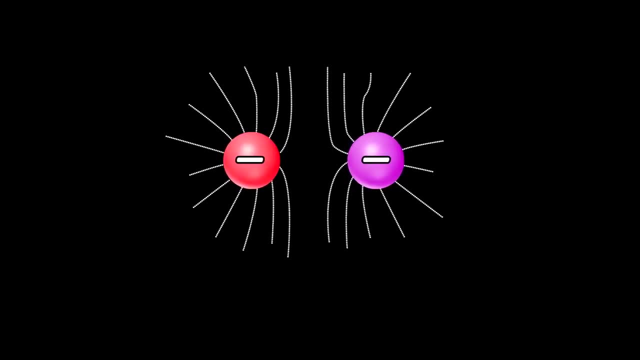 In classical theory, this would be thought of as the particles being repelled due to the interactions of a continuous field. In QED theory, however, the path can be simplified to look like this. 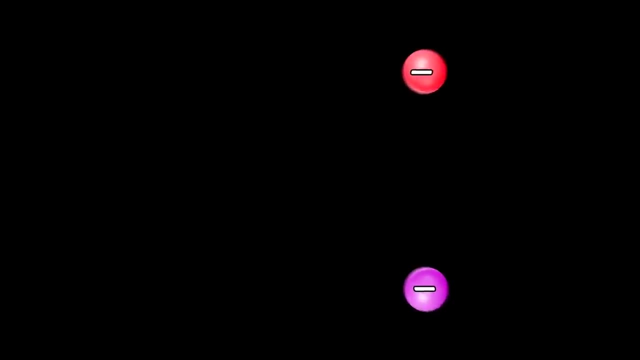 So, what happens here is that the two charged particles approach each other represented by the lines with the arrows moving towards each other. An exchange of a virtual photon takes place, represented by the wavy line in the middle. This exchange results in two charged particles moving away from each other, represented by the two lines pointing away from each other. 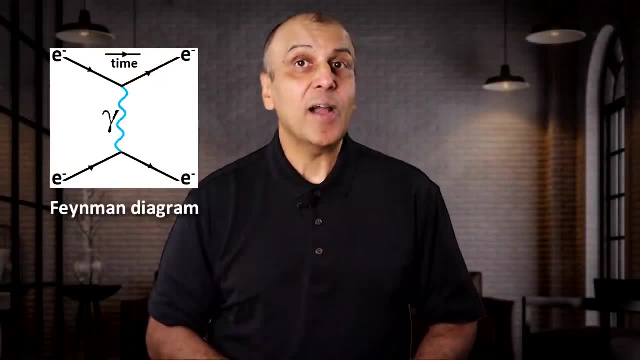 If you understand this, then you have just learned how to read a Feynman diagram because that's what this is, a simple Feynman diagram. 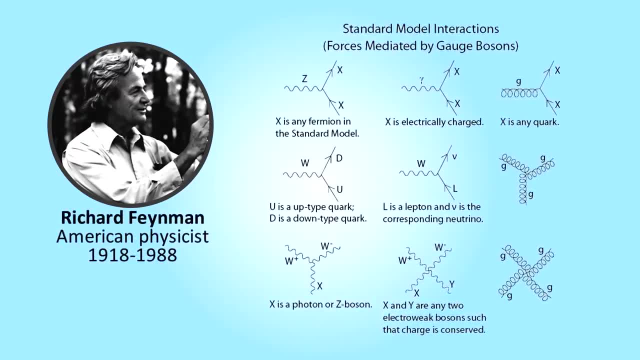 Feynman diagrams were developed by American physicist Richard Feynman around 1949 and 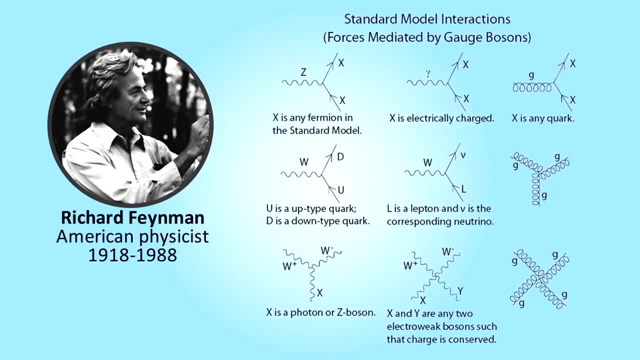 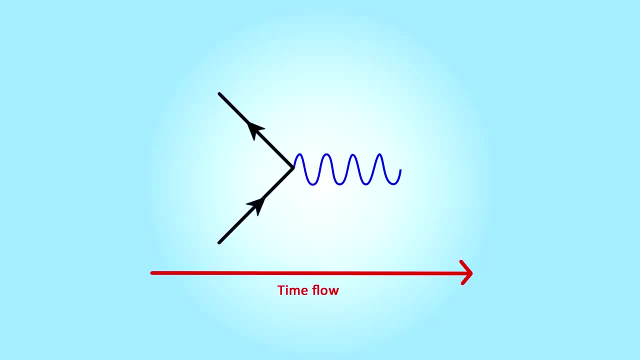 they help to intuitively understand the mathematics of QED. In more general terms, the simplest Feynman diagram can be drawn like this. The direction of the arrow of the fermion lines tells us whether the particle is a matter or antimatter particle. If the arrow goes forward in time to the right, it's a matter particle and if it goes backwards, it's the antimatter particle. So, in this diagram, the lower arrow pointing to the right represents the matter particle and the upper arrow represents the antimatter particle. This diagram can be interpreted as a positron and an electron annihilating into a photon. But we can also flip this 180 degrees and then the diagram would show a photon becoming an electron-positron pair. 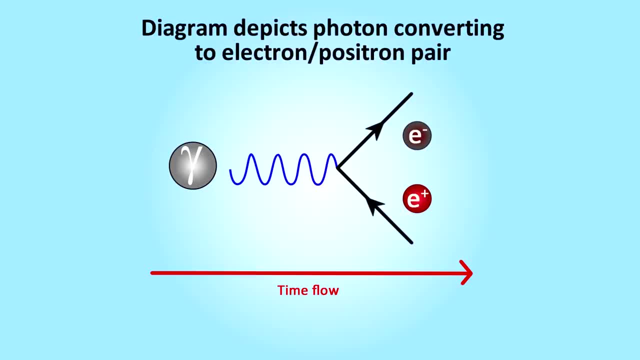 It turns out that from this simplest Feynman diagram you can build all other diagrams for QED. The lines with the arrows represent fermions and they must be continuous. 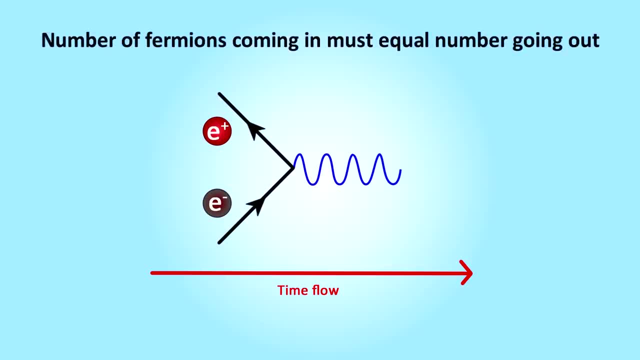 This is because of the law of conservation. The same number of fermions coming into a process must also come out. Note that a photon is a boson, not a fermion. 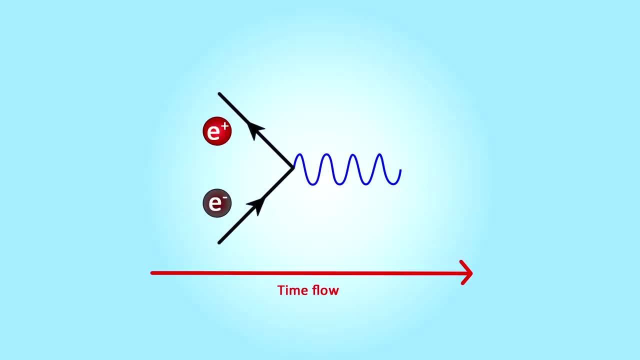 But you might ask, if a positron and an electron come in and a photon comes out, how are things conserved? 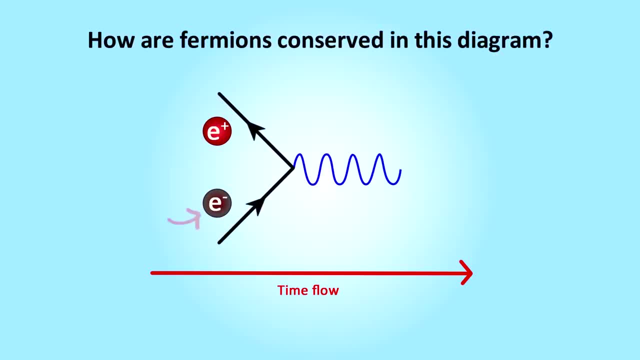 The reason conservation is still valid is because a matter particle is considered a plus one fermion and an antimatter particle is considered a minus one fermion. So, if 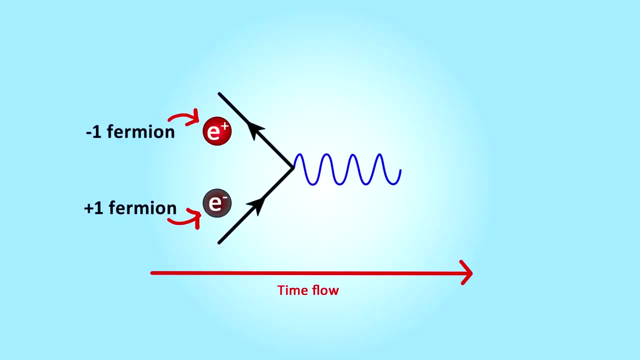 we look at the left side an electron and positron coming in works out to be plus one minus one which equals zero and then the other side there are no fermions. 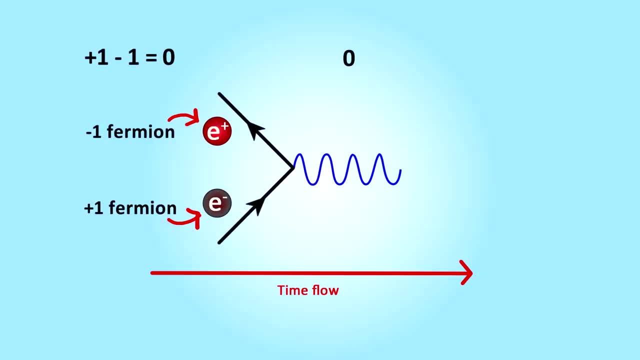 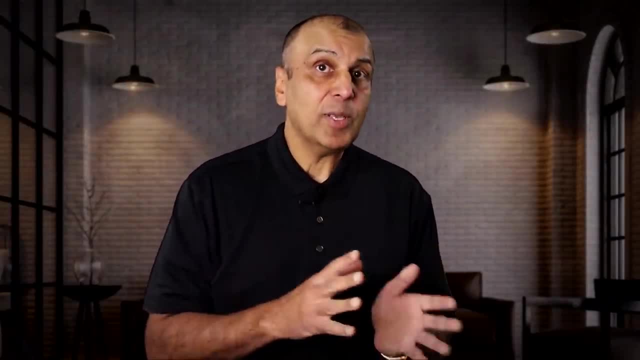 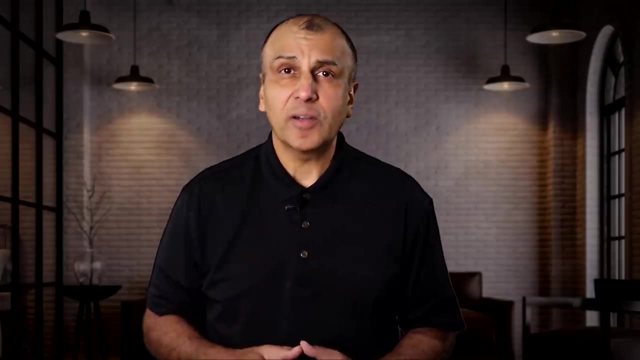 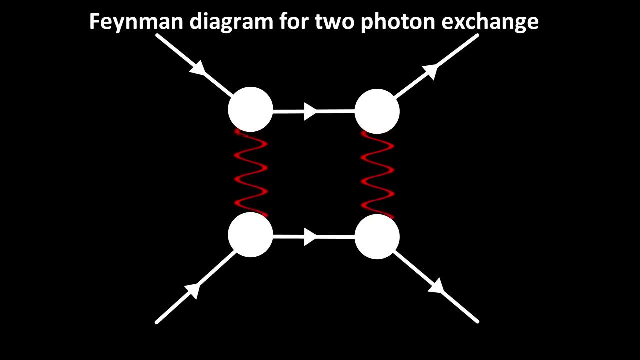 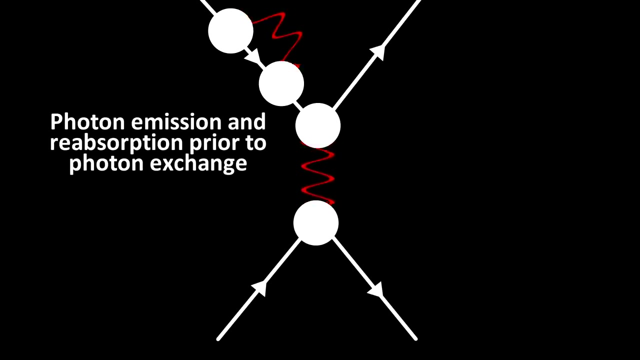 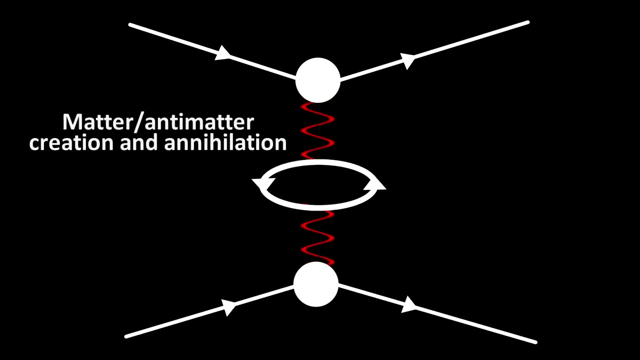 Thus we again have zero coming in and zero going out. The rule still works. Now you have to keep in mind that quantum theory is such that other events more complicated than the simple conversion to a photon or exchange of one photon can occur when two particles come near each other. So for example two photons can be exchanged. The Feynman diagram in that case looks something like this. Sometimes a particle can emit a photon and reabsorb it again before a photon exchange. The Feynman diagram for that looks like this. Since photons can carry various amounts of energy depending on their frequency, it can turn into a matter-antimatter particle. For example electron-positron, muon-antimuon, quark- antiquark during the exchange process and the diagram for that occurrence looks something like this. 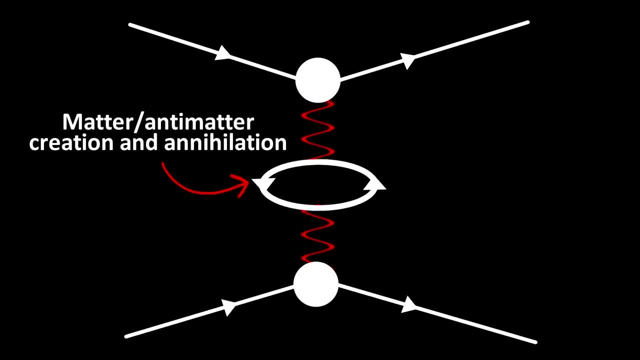 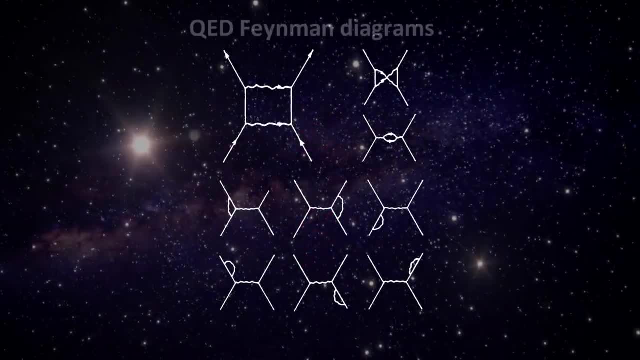 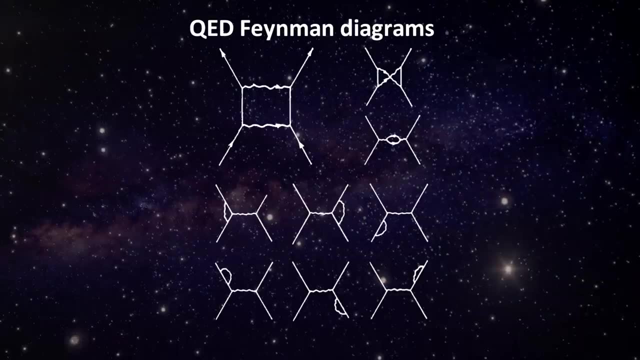 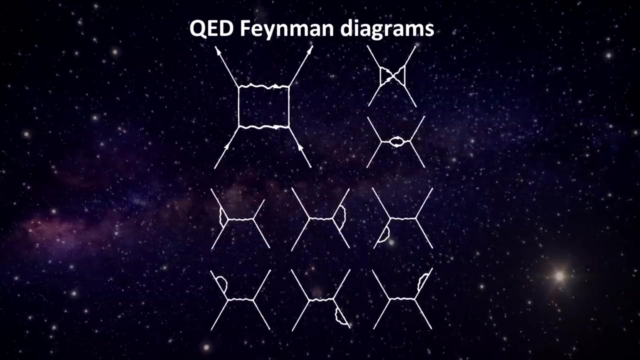 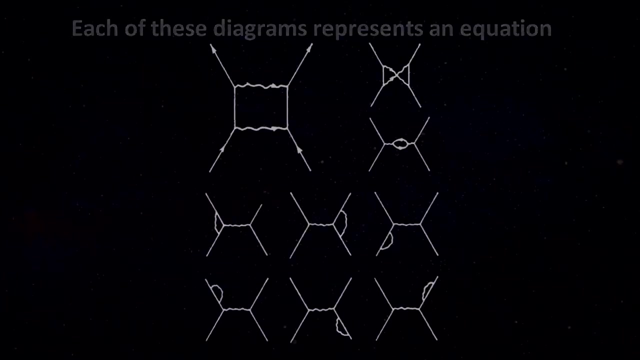 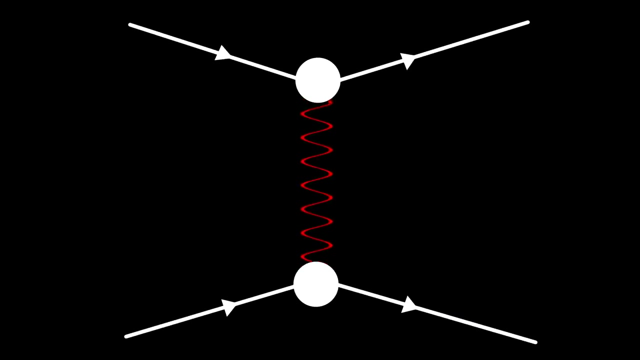 The fineman diagram in that case looks something like this. The fineman diagram represents matter-antimatter creation and annihilation resulting in a reconversion back to a photon. Just about anything can occur in these interactions so we can have all kinds of diagrams here. The key to understanding Feynman diagrams and the brilliance of Richard Feynman is that he was able to develop an intuitive pictorial representation of highly sophisticated mathematics because you see every one of these Feynman diagrams is really an equation, a rather complicated equation. So for example in one of the simplest diagrams where two electrons come in and two electrons come out and a photon is being exchanged, this equation has seven components. The two electrons coming in, two electrons coming out, a photon being exchanged and a vertex where the photon is emitted and a vertex where the photon is absorbed. Each of these seven components has an associated element in an equation. So using these components we can write the equation and it looks like this. This is the mathematical equivalent of the same simple Feynman 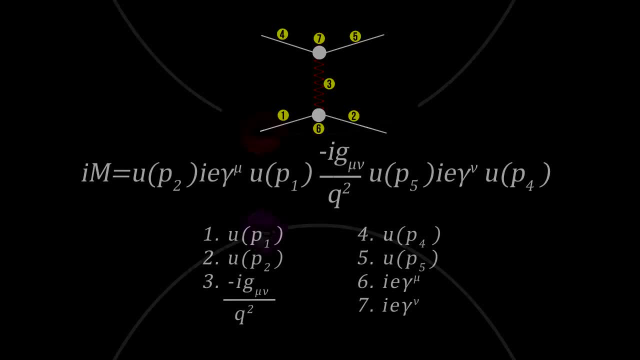 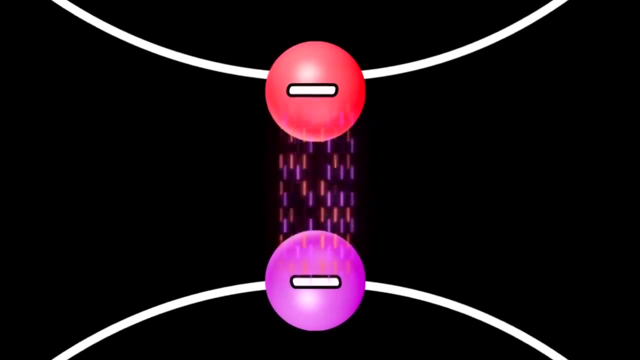 diagram. Note that when two charged particles actually come near each other they exchange many photons, not just one photon, and many different types of potential exchanges can occur. But by simplifying the equation to the exchange of a single photon we can get a pretty good approximation of what's actually 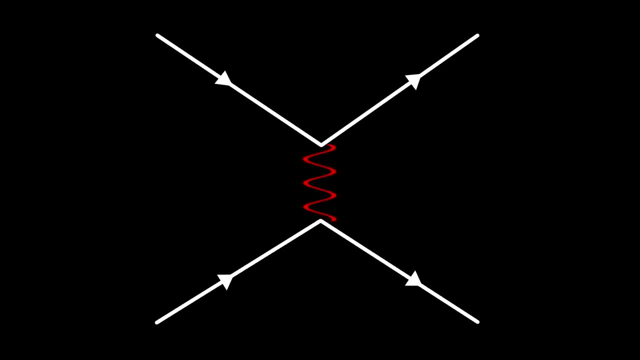 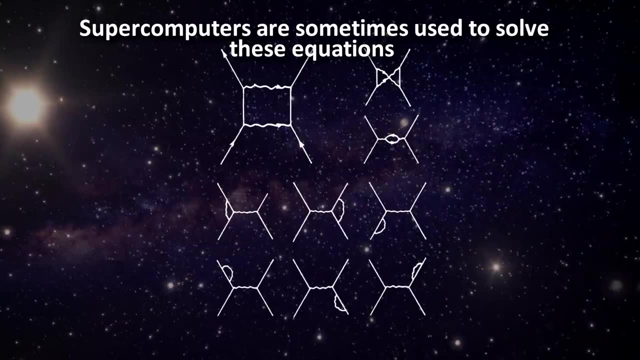 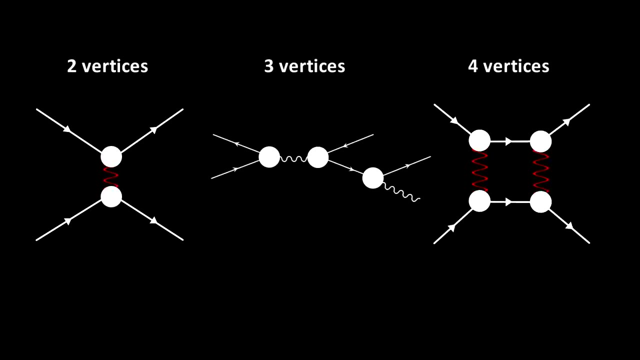 happening and that's what makes these Feynman diagrams so useful. Multiple components and multiple vertices can quickly result in very complicated equations but solving them is a whole different story and sometimes supercomputers are used to solve them. We can also calculate the probability of any one of these Feynman diagrams. It turns out that the probability depends mostly on the number of emission and absorptions. And an emission and absorption on a Feynman diagram is shown as a vertex. The more vertices the less 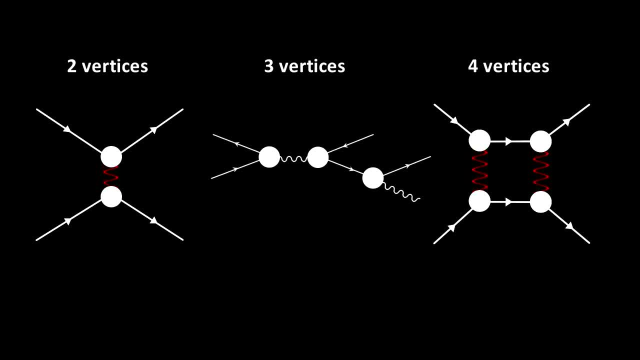 likely it is to occur. Each vertex on a diagram means that it happens 1% as often as a diagram with one less vertex. So for example, a diagram with three vertices happens 1% as often as a diagram with two vertices. Four vertices happen 0.01% as often as a diagram with two vertices. One